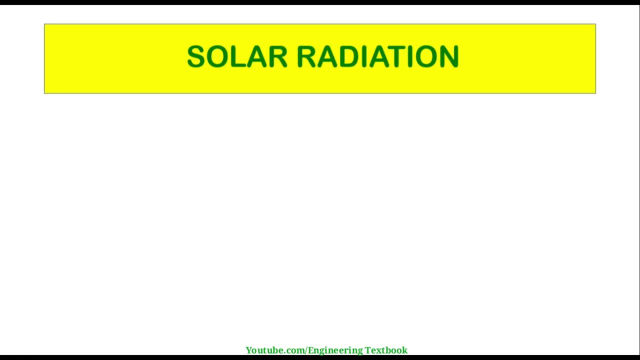 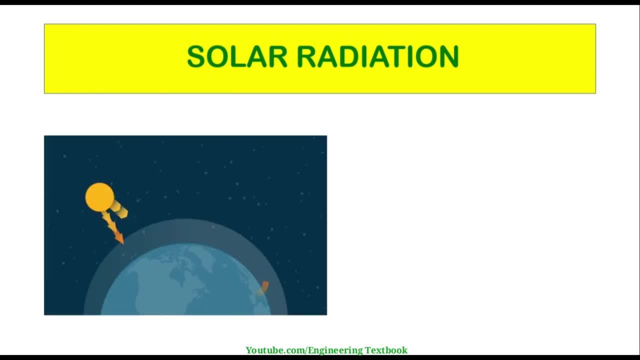 Hello everyone, welcome back to my channel. So today's video is about solar radiation. Solar radiation is the energy emitted by the sun through electromagnetic waves, and life on the earth depends upon it. In addition to determine atmospheric and cinematographic dynamics and trends, it makes plants photosynthesis possible, among other processes. 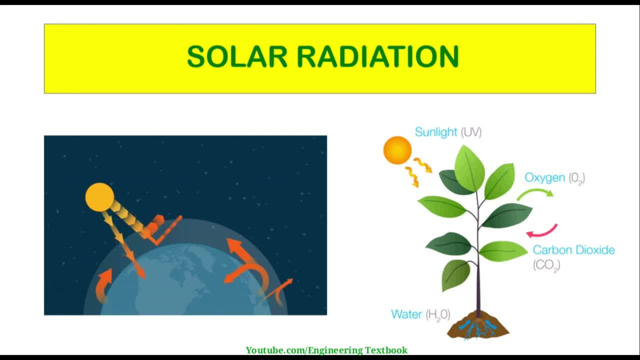 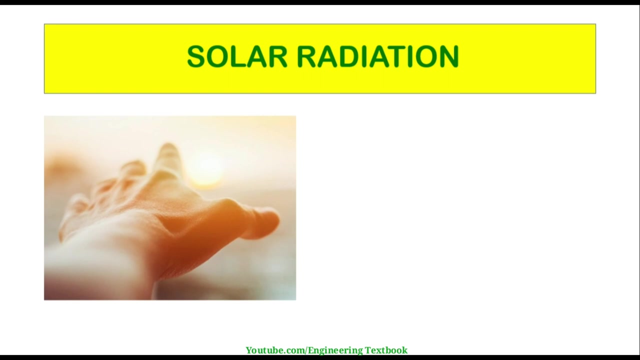 Without solar radiation, there would be no life on the earth. Moreover, it currently allows us to produce photovoltaic energy, which is essential in the fight against climate changes. However, it can also be harmful to human life, For example, due to its effect on our skin. and this effect. 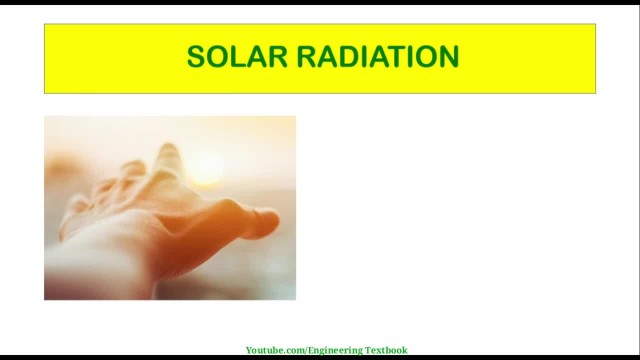 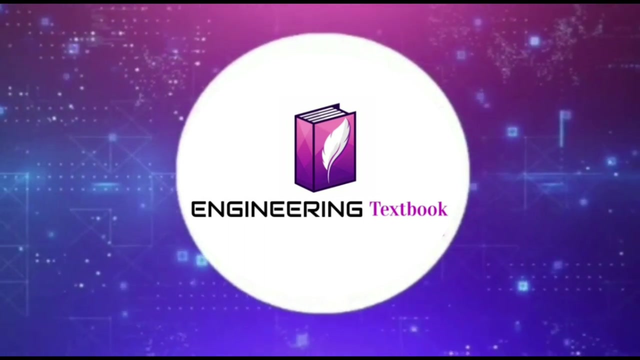 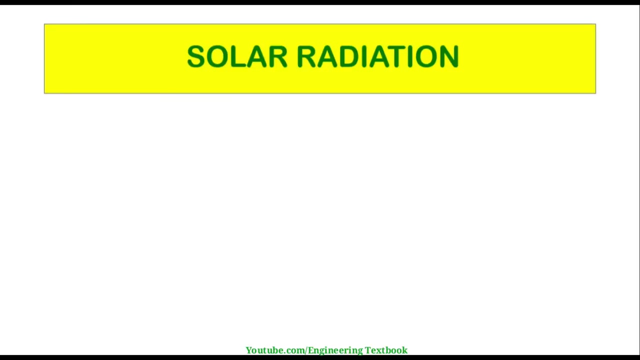 have become more dangerous in reality In recent year due to greenhouse effect, which also influence the rising temperature of our planet. So in this video we will study about solar radiation, its types and how it is measured. So let's see the definition of solar radiation. 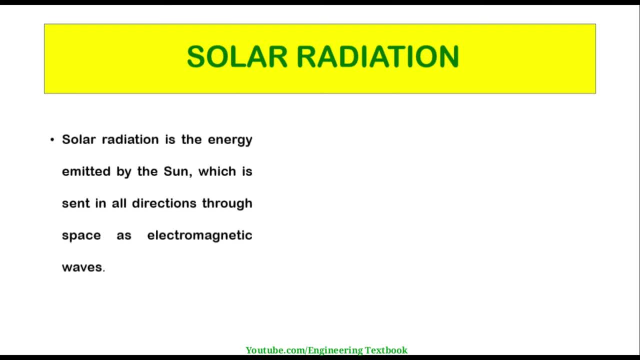 Solar radiation is the energy emitted by the sun which is sent in all directions through space as electromagnetic waves. So it says that the energy emitted by the sun influences atmospheric processes. It is also directly and indirectly responsible for common phenomena such as plant photosynthesis. 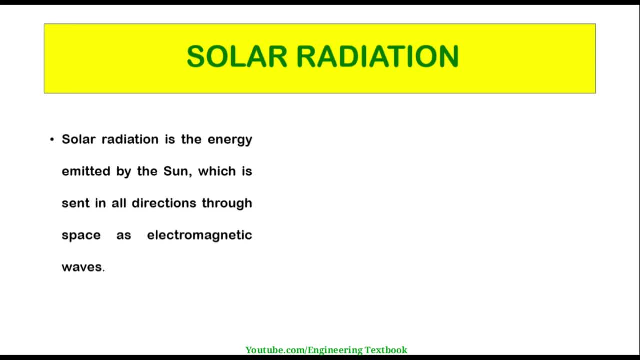 climate changes, temperature, temperature of living space, energy present in the atmosphere. energy in the atmosphere, Then, it is also responsible for generating direct and indirect energy. Here in the figure, we see the sun emitting energy in the form of short wave radiations, which is weakened in the atmosphere by the presence of electromagnetic waves. 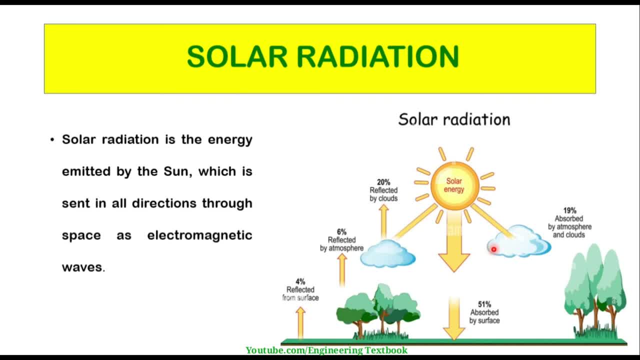 The sun emits energy in the form of short wave radiation, which is weakened in the atmosphere by the presence of electromagnetic waves loud and absorbed by the gas, molecules or suspended particles present in the atmosphere. after passing through the atmosphere, solar radiation reaches the continental land surfaces and is reflected or absorbed. 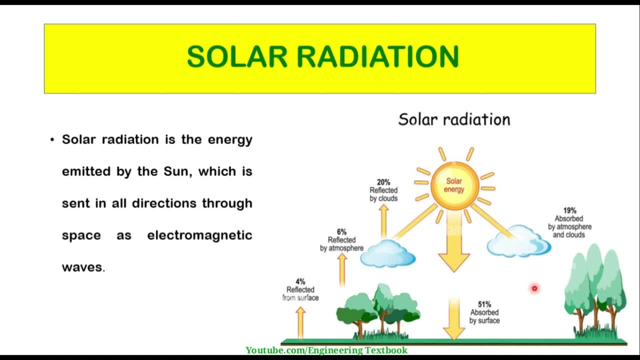 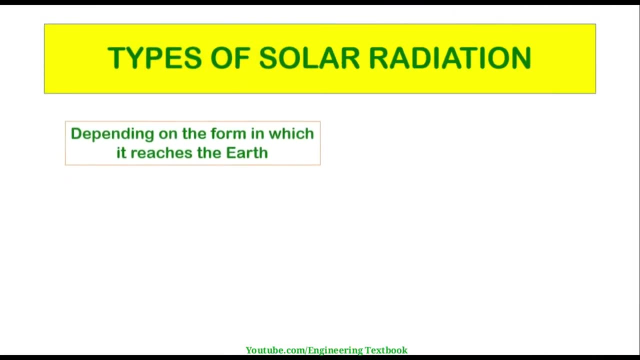 finally, the surface returns it to the outer space in the form of long wave radiations. types of solar radiation: depending on the form in which it reaches the earth's surface, there are three types of radiation. first is direct solar radiation, diffused solar radiation and reflected solar radiation. let's see in it in detail. 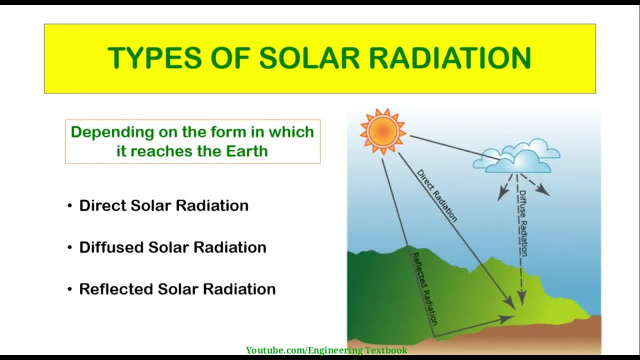 this figure shows all the types of solar radiation that are present in the atmosphere. there are three types of solar radiation. in detail here we see direct radiation, diffuse radiation through clouds and reflected radiation reflected over the surface. so direct radiation reaches the earth surface without disappearing at all on the way. 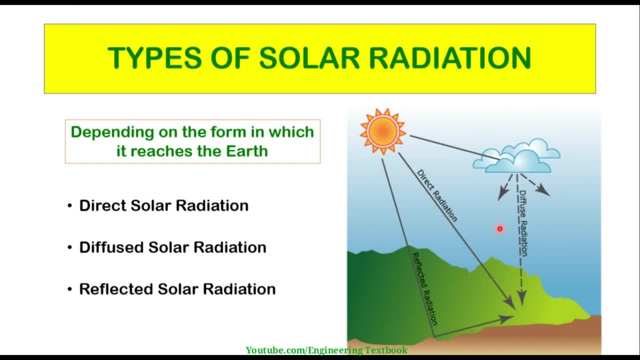 that is, it does not change its direction. it reflect on the surface directly. Next is diffuse radiation. Diffuse solar radiation reaches the earth's surface after having undergo multiple deviation in its trajectory, for example clouds or gases, presence in atmosphere, etc. So diffuse radiation changes. 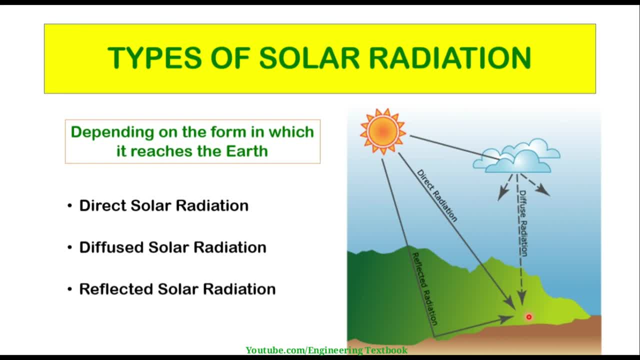 the direction, and then it is radiate on the surfaces. Next is reflected radiation. Reflected solar radiation is fraction of solar radiation that is reflected by the earth's surface itself in a phenomena known as ablando effect. So it states that it first radiates on the 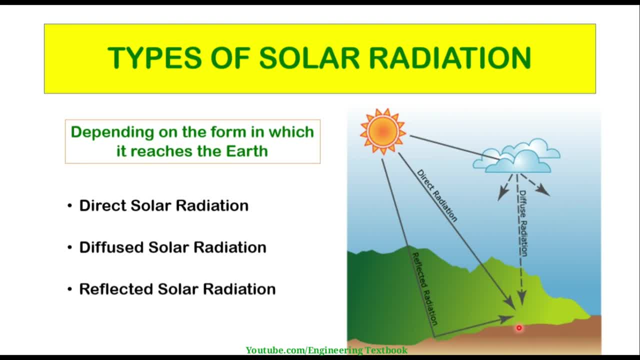 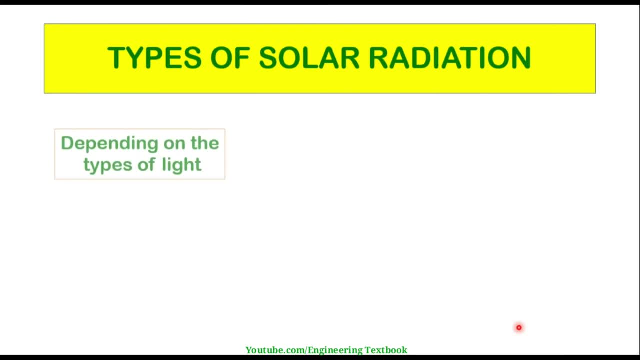 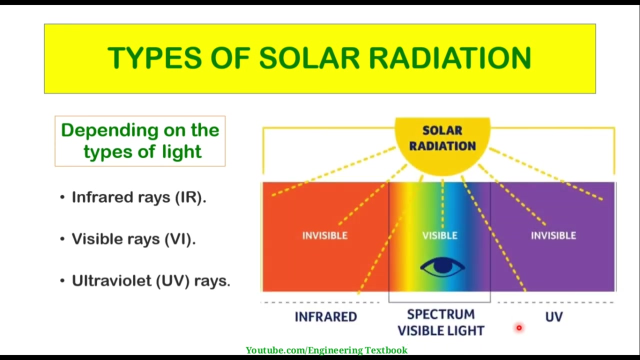 surface and reflected over the surface is known as reflected solar radiation. The next is depending on types of light. there are again three types of solar radiation: Infrared radiation, visible radiation or rays, ultraviolet radiation or rays. So this figure explains about these three types of radiations: Infrared rays spectrum. 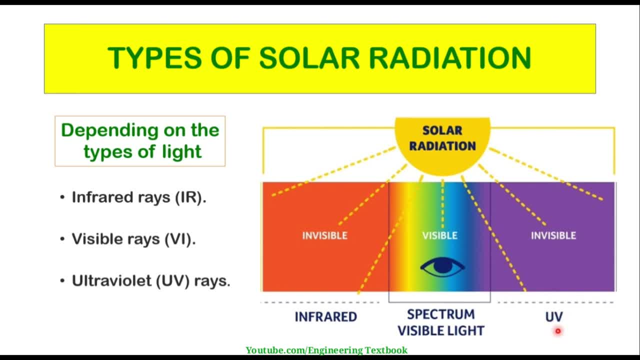 or visible rays or light, UV. UV means ultraviolet rays. It is also known as invisible, visible, invisible solar radiation. So let's see it: Infrared rays, long-term radiation, visible light and dark wave length. They emit heat and are given off by anybody. those temperature? 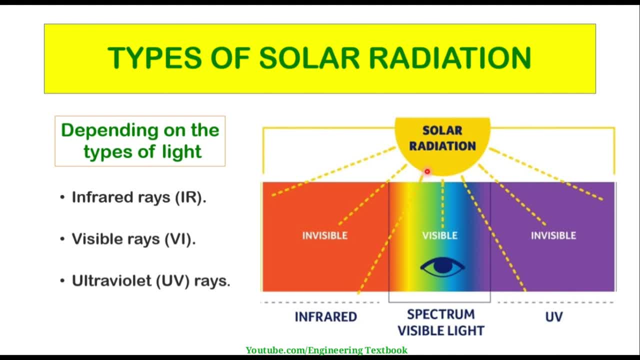 is greater than 0 degree Kelvin. So the solar radiation which temperature is greater than 0 degree Kelvin is known as infrared rays, and it is not visible to the human eye. Visible rays- visible rays- as if the name suggests that light is visible in the sky. 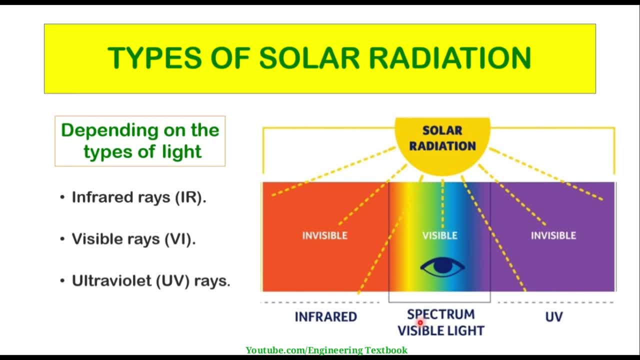 suggest it is visible to the human eye. it is also known as spectrum rays. they emit the light and those that a human eye perceive in the form of color, that is, we can see these rays in the color red, orange, yellow, green, blue or violet. these color rays are known as visible rays. 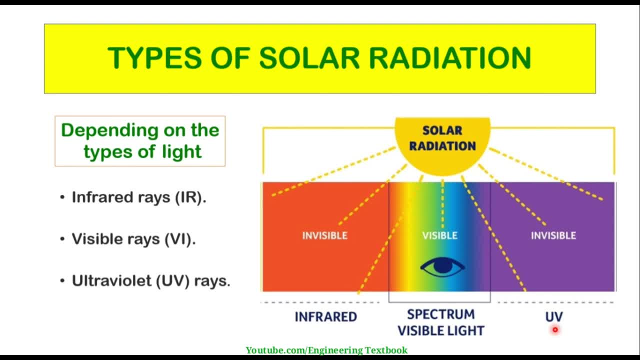 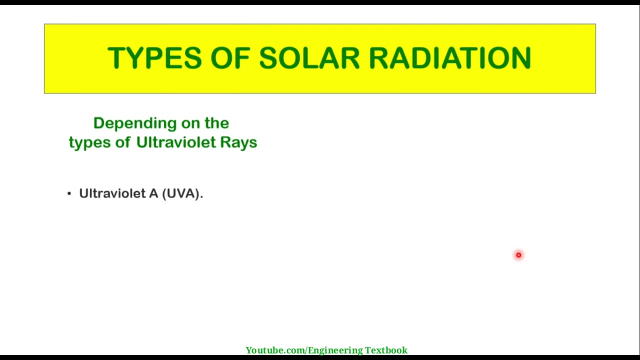 ultraviolet or uv rays. they are invisible to the human eye and have more serious impact on the skin. they are divided into three subcategories. so this uv rays are also known as invisible rays and are again divided into three categories. they are ultraviolet rays a- uva, ultraviolet rays b- uvb and last is ultraviolet rays c- uvc. 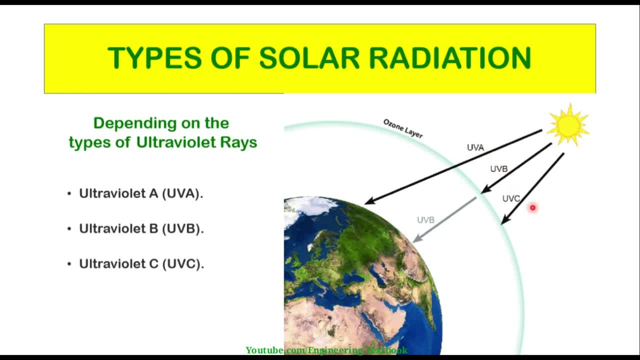 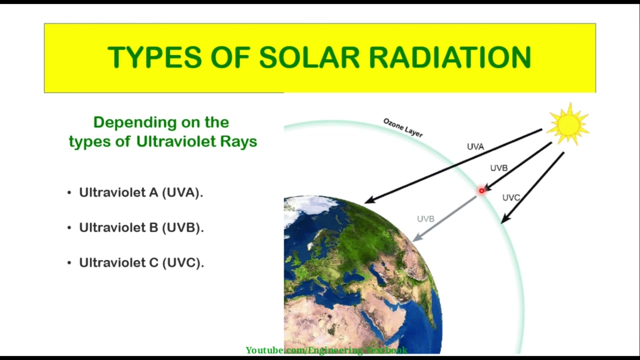 this figure explains about three types of ultraviolet rays. the ultraviolet light passes through the atmosphere easily, most of it reaching the surface of the planet is known as ultraviolet ray a. the ultra violent light rays, does not penetrate to the atmosphere so easily. even so, it reaches the surface. 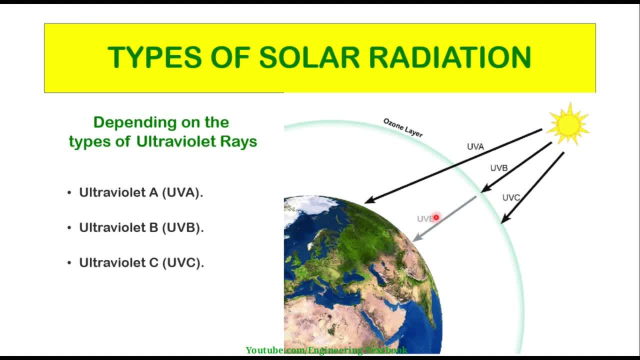 and is responsible to worse skin damage, is known as ultraviolet rays b b. the ultraviolet light is responsible to worse skin damage is known as ultraviolet rays b- uvb. that cannot get through atmosphere so easily because it is absorbed by the ozone layer present here, so that race is known as UVC- ultra-violet rays, see. 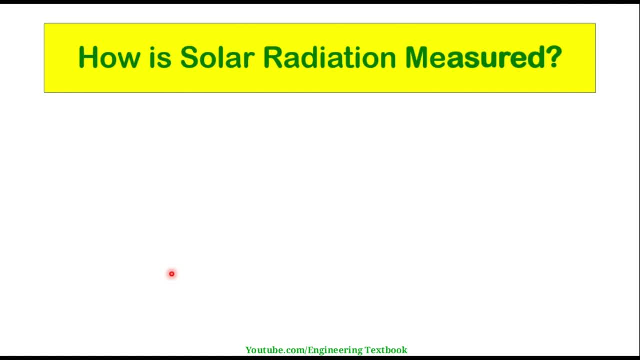 you. next is: how is solar radiation measured? solar radiation is measured on a horizontal surface by means of radiation sensors or pyranometer, which is placed in south-facing shadow. pre-location data are collected in. data are collected in units of power, so the solar radiation unit is Watt per square meter. 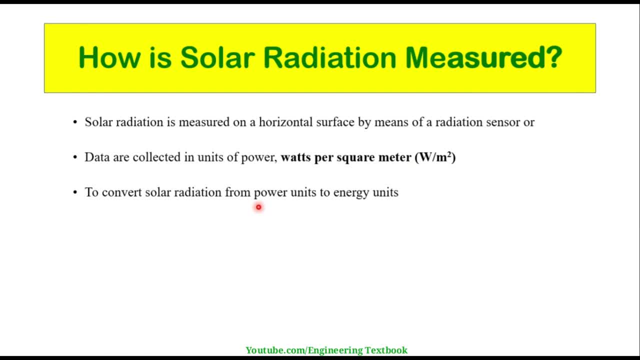 to convert solar radiation from power unit to energy unit, the data in Watt per square meter must be multiplied by the number of seconds compromising, that is 600 seconds, or 24 hours, that is 86,400 seconds, and the result will be provided in joules per square meter. so here it states that, if you want,